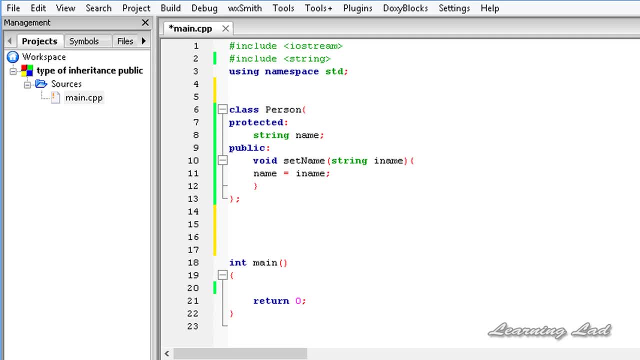 Hi, this is Anil and welcome to the video tutorial for the learning lab on C++ programming. So in this tutorial we gonna learn about the type of inheritance. So when we derive a class from a base class, you know we used to specify the access specifier as public, private and protected. So when we use the specific access specifier, you know, while deriving from a base class, you know that access specifier is gonna have a certain impact on the learning lab. 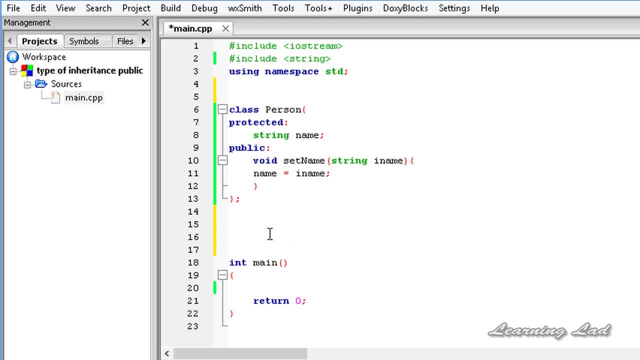 On the behavior of the base class members in the derived class. So if it is confusing, don't worry. you know, when we see the example it's gonna be clear. So here in this tutorial we gonna learn about the public inheritance. A public inheritance is nothing but using the keyword public while inheriting from a base class. So here, for the demonstration purpose, I have a class called person. You know, this class is gonna act as the base class in our program And as a product. 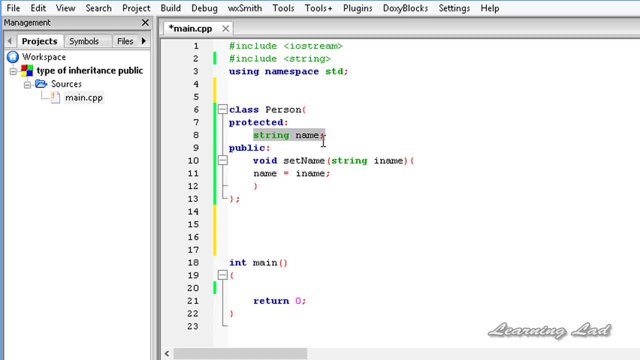 member. I have a member called name and as a public member, I have a method, you know, which is gonna initialize this protected member name. Alright, now I'm gonna build a derived class called student, and this student is gonna be inheriting from this class person. So here we gonna use the access specifier as public, So this type of inheritance is called public inheritance. So when we use the 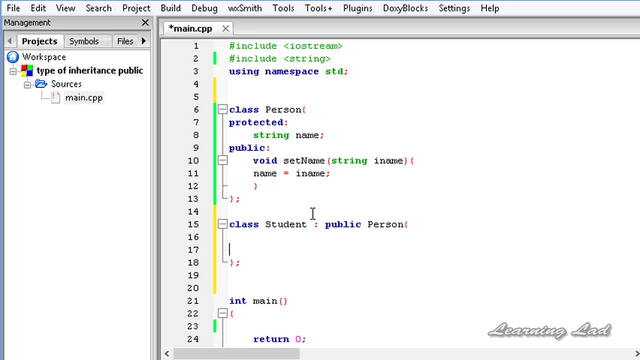 public inheritance. you know which is the most commonly used inheritance type. you know all the public members of this base class are gonna act as the public members of this derived class And also all the protected members of this base class are gonna act as the protected members of this derived class. And if we have any private members in the base class, you know they are not available in the 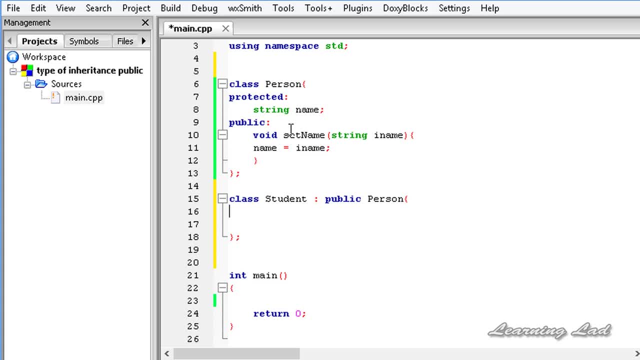 derived class. So now here in our program, you know, this protected member name of this base class will acts like a protected member of this class student and the public method of this base class person, which is set name, is going to act as the public method of this class student. so just to demonstrate that, 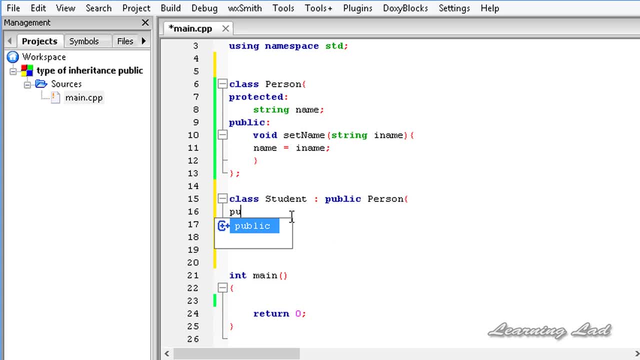 here in our tutorial. let's build a quick method. let's have access specifier public and this method is going to display the value of this member name, so it's going to be void display. you guys can give it any name and we're going to use c out and it's going to be name and let's 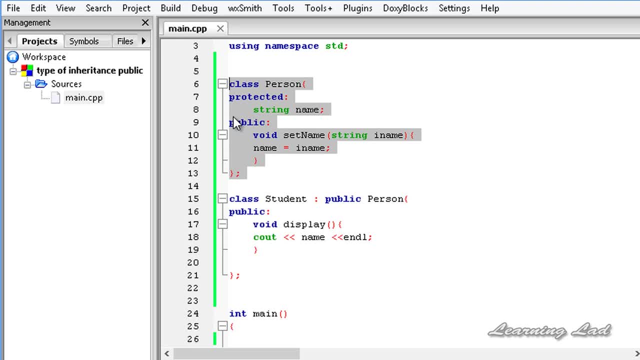 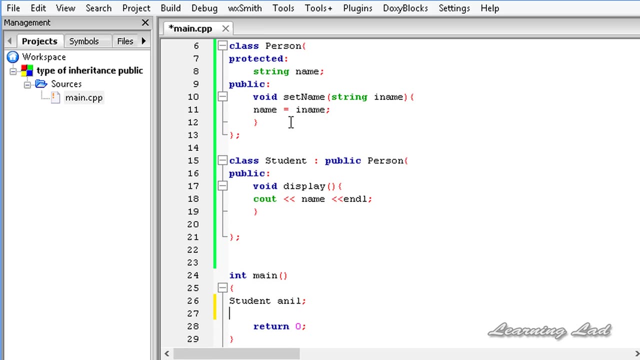 end this line. all right now. we have a base class called person and we have a derived class called student and we have the public inheritance here. all right now, let's create an object of this class: student. so it's going to be student and anil, now the public. 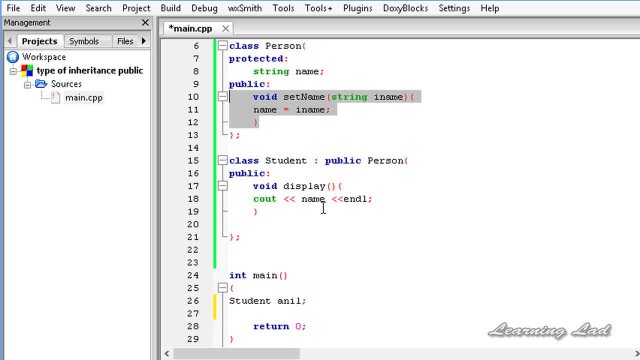 member of this class person or the base class is going to act as the public member of this derived class or the class student, and that's why we can access this public member outside this base and the derived class. that's why i can access anil dot and then the set name. so let's set a name. 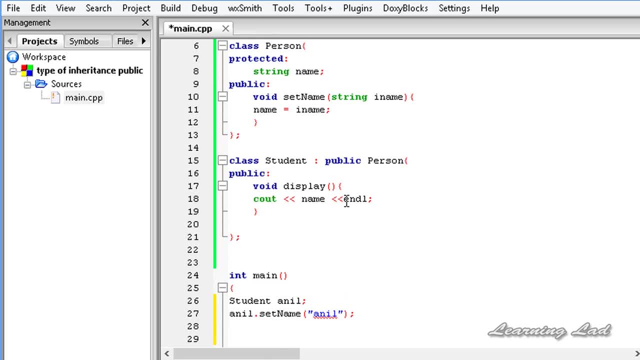 and then we have the public member of this class student. we can access that. so it's going to be anil dot display and let's save this. let's build and run this program, just to make sure that it's working properly. all right, we got anil. now you know this protected. 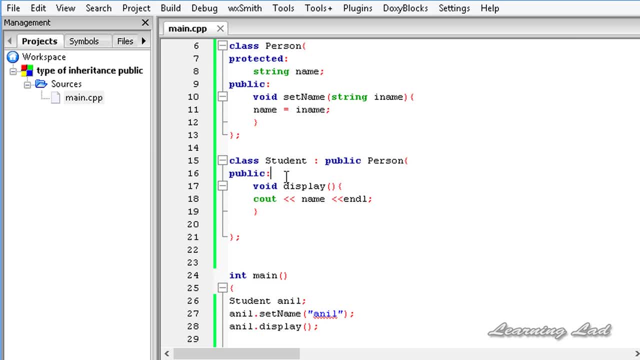 member of this base class person is going to act as the protected member of this class student when we use public inheritance at that time. you know, this name is not available outside from this derived class. so if we have any other class which is inheriting from this class student, then this name can be available in that. 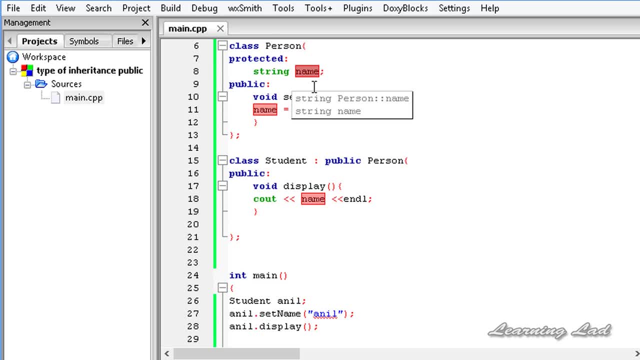 class. but you know this name is not available outside this base class or the derived class. that's why if i try to access that name here- anil dot name- and if i set to some value let's say ani, you know it is not possible and it's going to produce the error. so i'm going to build and run.